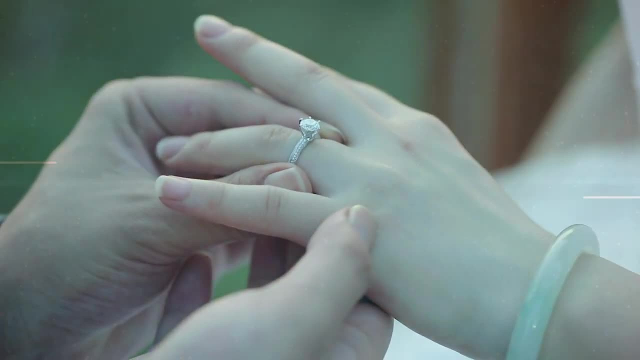 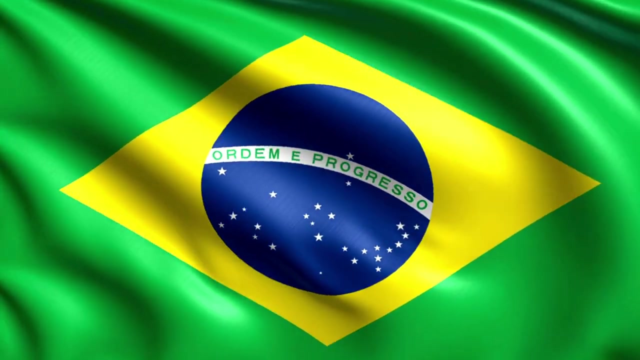 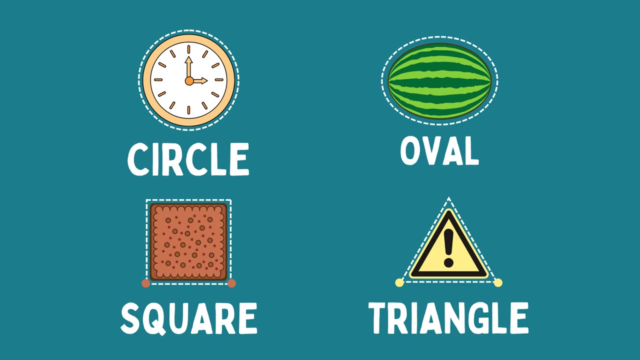 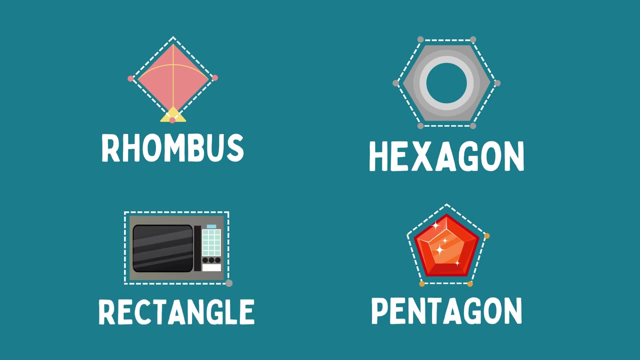 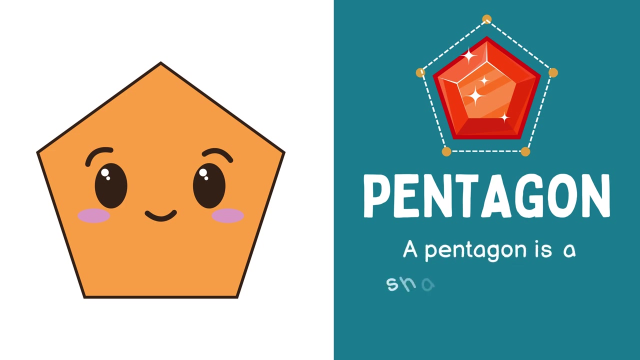 Remember today, Care of all young men and girls, Where you'll be one, yes, other than me, Itónme You so feel, Giga, Giga. That's it, St zg Giga. Let's learn them all, night by night. Let's explore the pentagon. 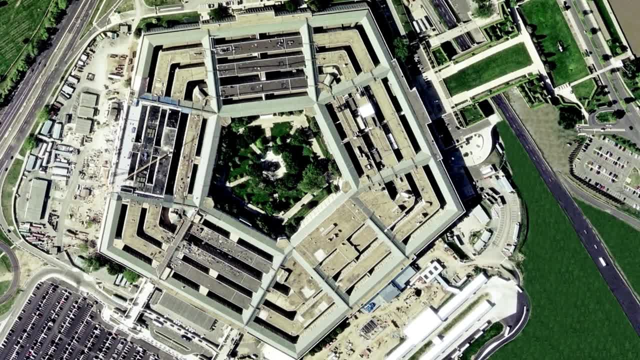 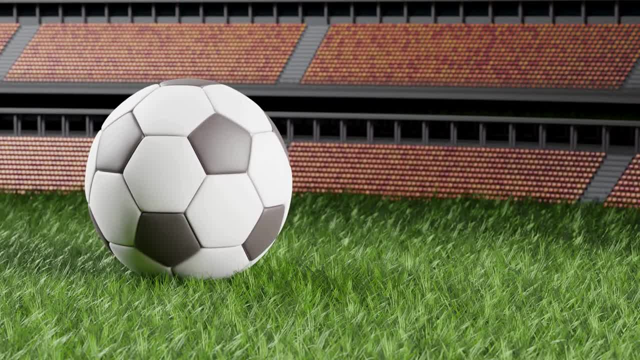 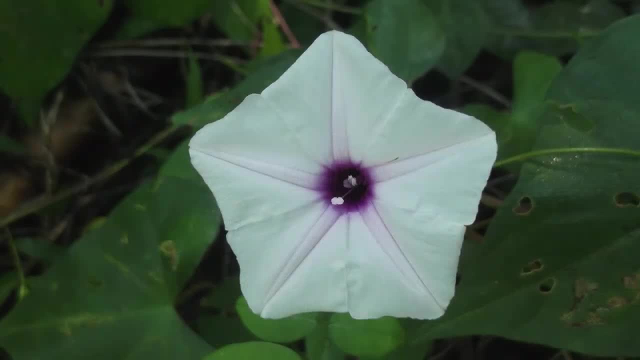 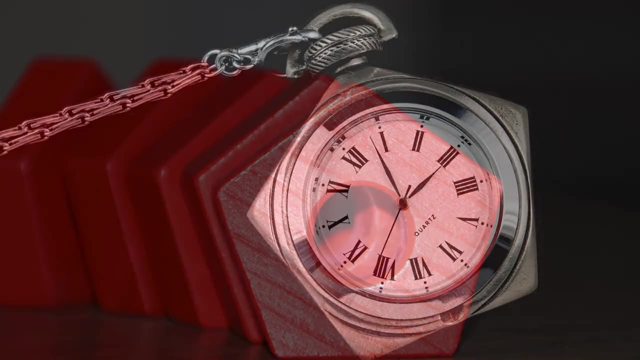 With five sides that stand strong and tall, A star-like shape with angles wide In geometry's grand hall, Each side unique in its length, Five corners where lines converge With five angles. you command attention In shapes that disperse From only on a baseball field To a pentagon shaped as outside an eel. 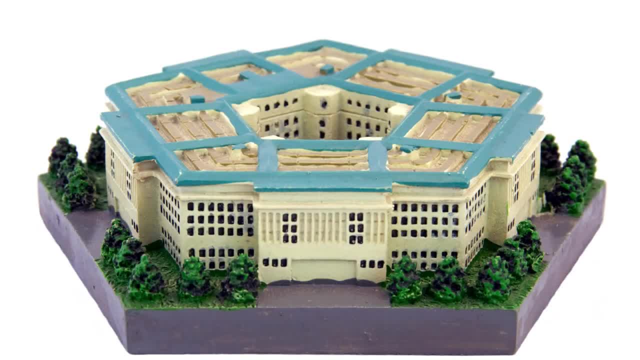 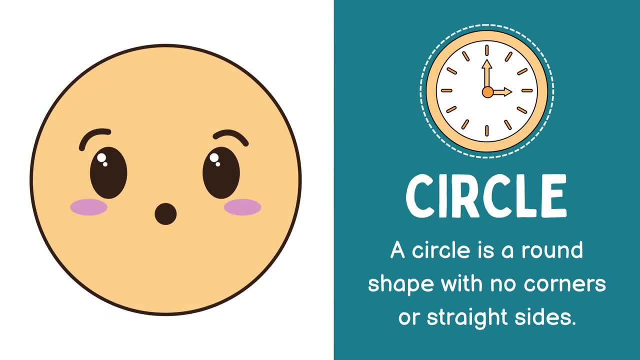 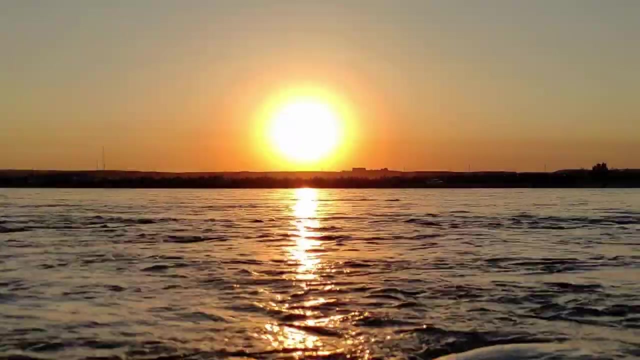 A pentagon's presence, an endless seal In symmetry, it wheels. Now let's circle back to the beginning, With a shape that's perfectly round, No coins to define, no straight sides in sight, A circle forever unbound, Infinite points along its edge. No beginning, no end. it's true. 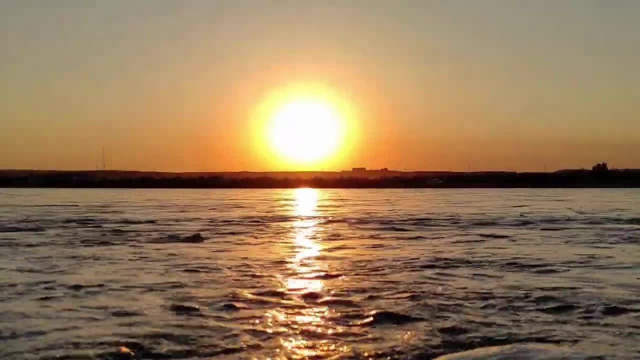 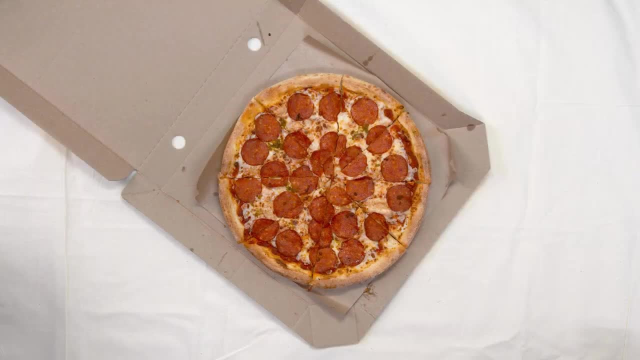 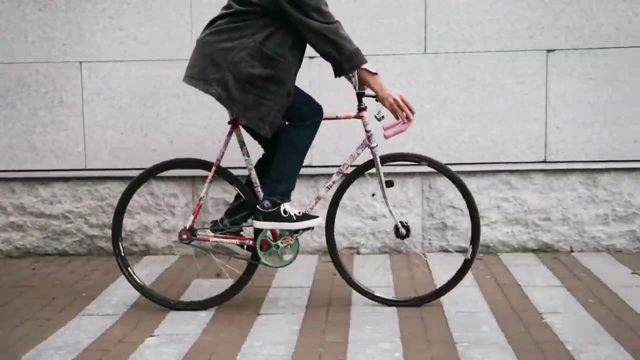 A wheel in motion, a ring of devotion In geometry's grand view From the sun in the sky To a piece of high, view From the sun in the sky To a piece of high, To the wheels on a bicycle ride, A circle's embrace so vast and wide. 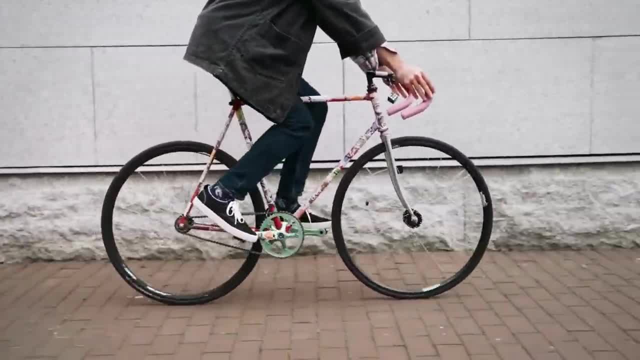 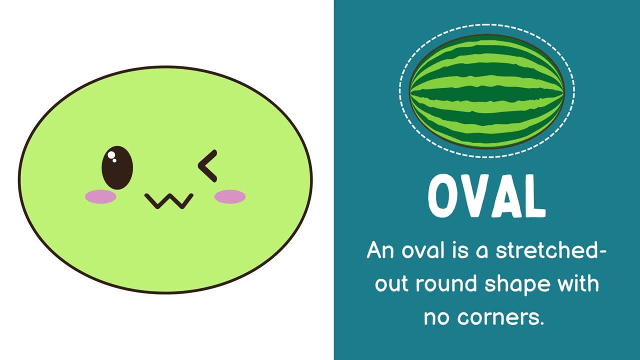 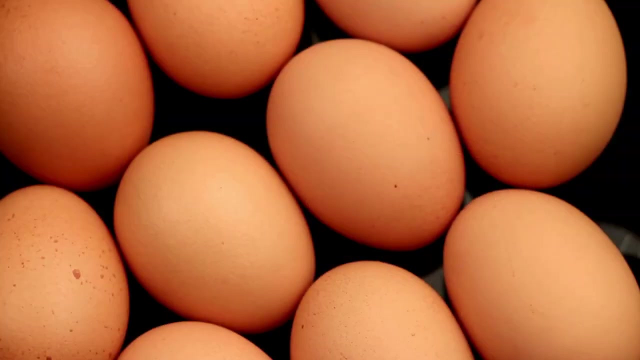 It's in a triangle shaped as outside, an eel. In symmetry it takes pride. Let's talk about the oval, A shape like a circle, But stretched and long, No corners to be found, Smooth and curved. In symmetry it belongs A stretched out ground. It gracefully flows In shapes. it holds a special grace. 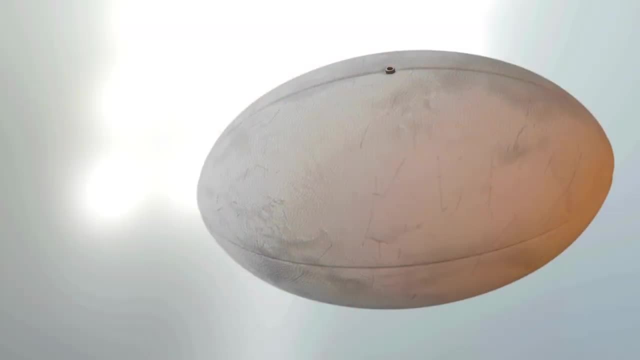 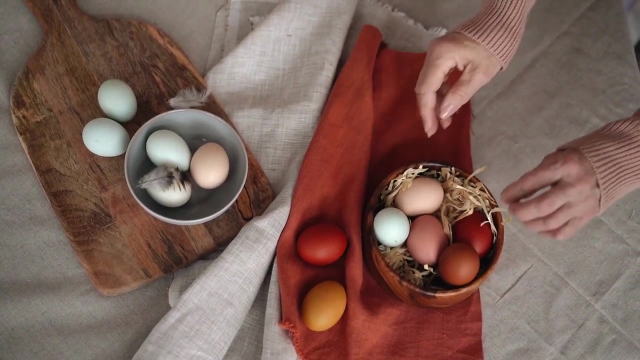 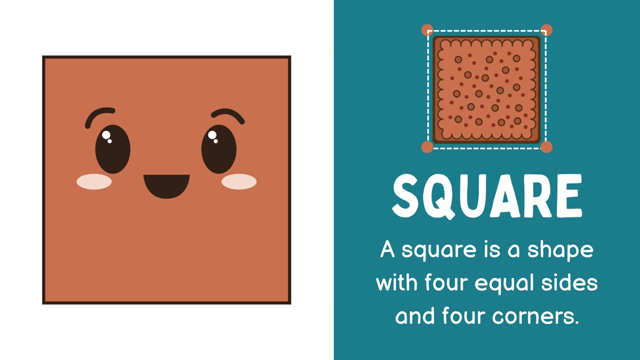 From made to the best To a rugby ball's quest. In ovals there's an embracing space With two symmetrical ends. it bends In symmetry. it gently extends The oval's charm. it transcends In shapes. it gives me a mess. Now let's square up. We're square up to the channel right. 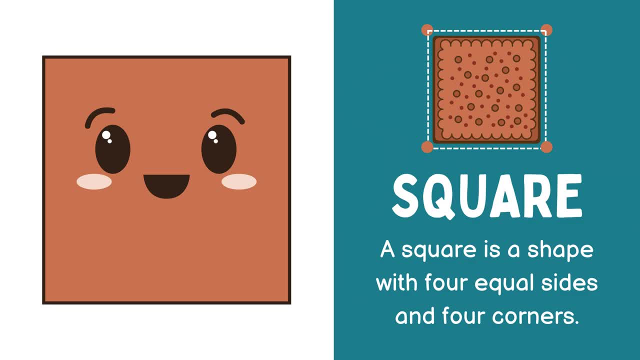 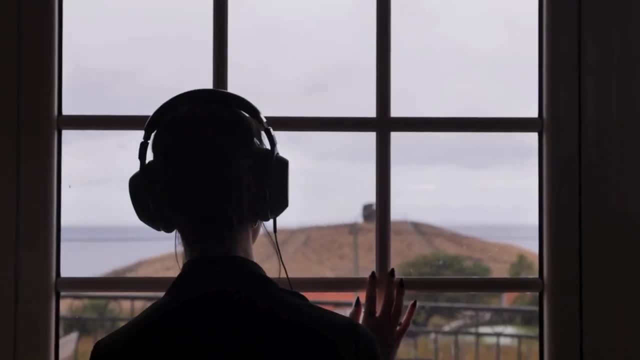 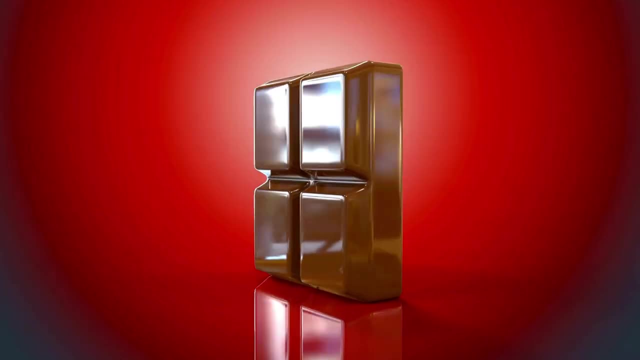 In symmetry it comes through. Four equals have the perfect match Like dots stacked in a circle So many growing times on the floor, In windows and doors. In symmetry It's beauty to show From a gift-wrapped box To a chocolate bar, To a windowpane watching a farm. 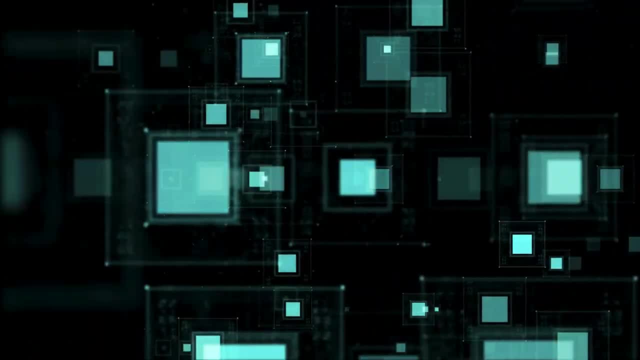 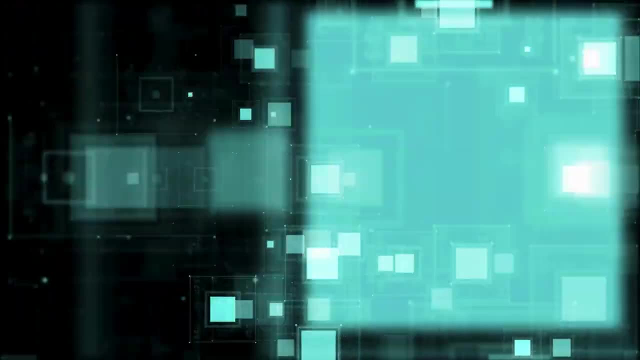 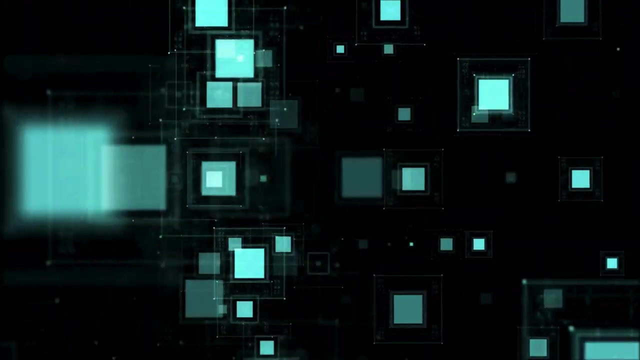 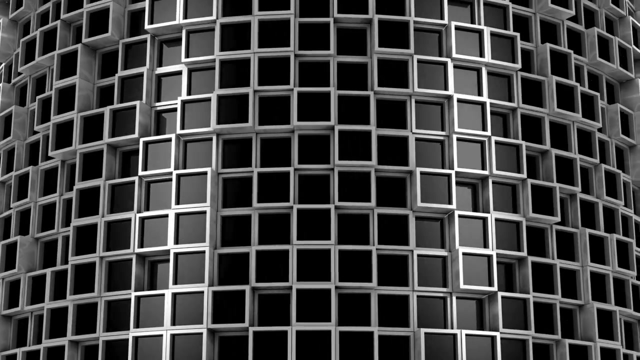 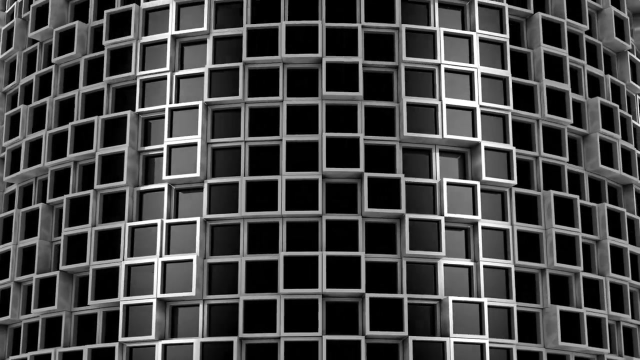 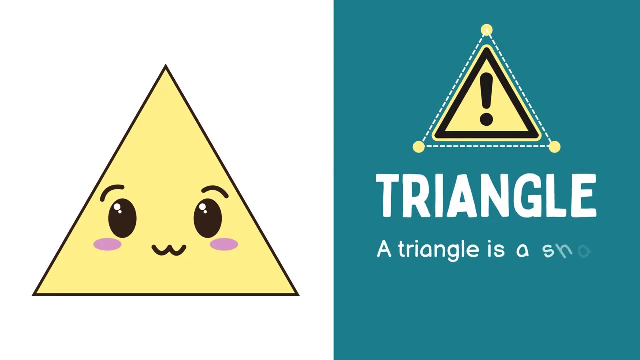 A square's simplicity, A guiding star. In shapes it's as familiar as a tongue. So if that box to a chocolate bar, To a window pane watching a far, The square, simplicity, a dining star, It shapes itself. Now let's delve into the triangle. With three sides it stands bold and strong. 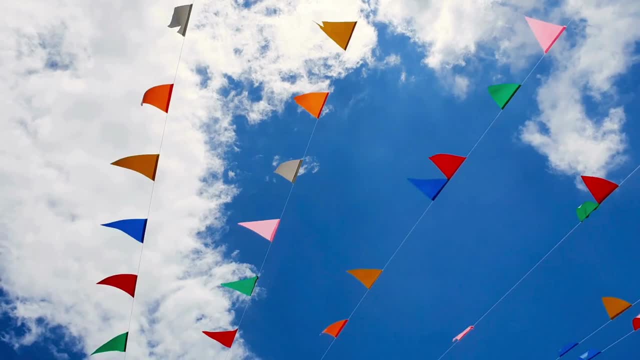 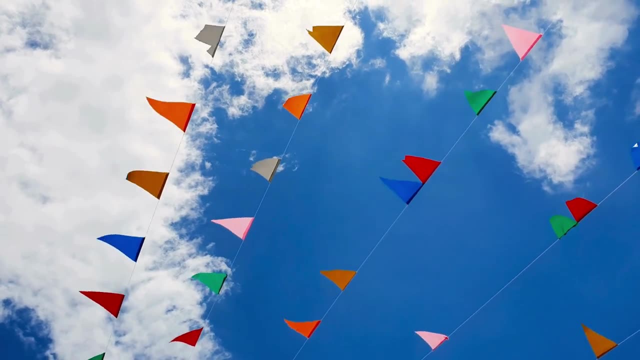 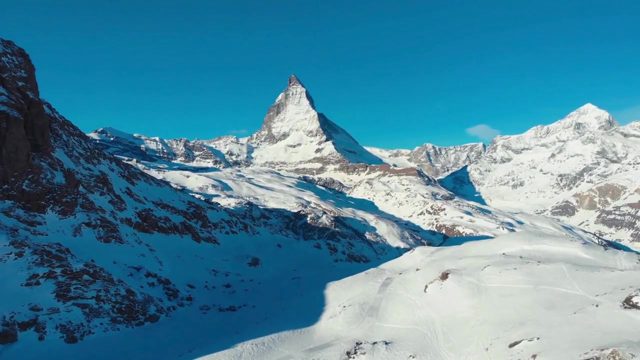 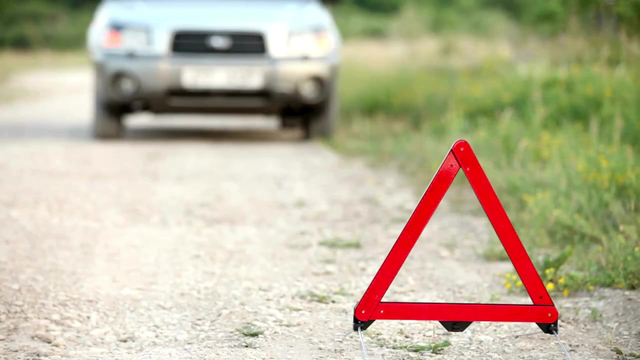 Three corners where life's converging Geometry spans on each side A unique length. it holds Three corners, each with its tail, From pyramids spread to flags in hand. In triangle, stories prevail In mountains high in sails. sails unfurl In arrows pointing to the world. Triangle shape forever slow. 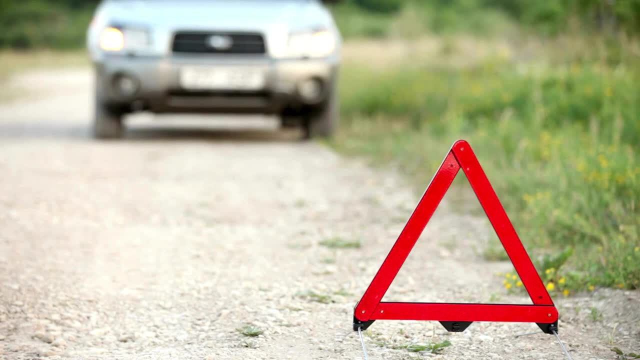 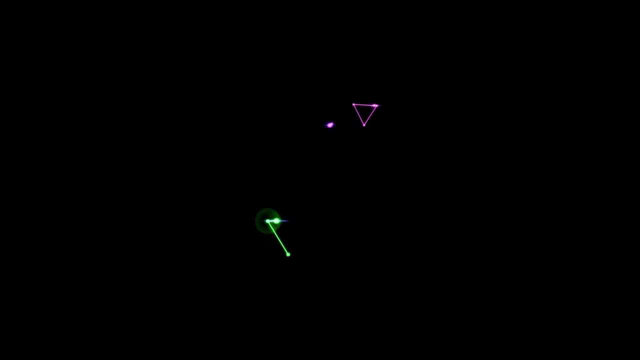 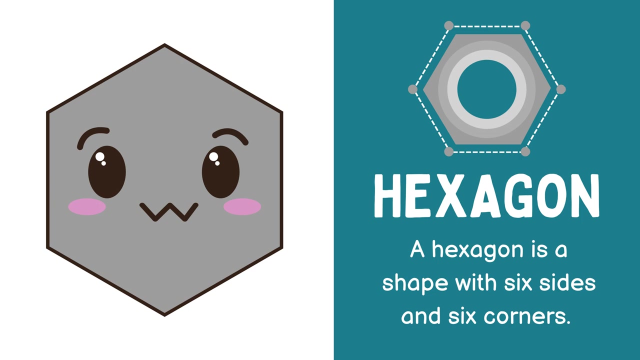 In symmetry, it's unfurl. Next in line, its targets are gone. With six sides, it's a marvel to behold Six corners where life's converging Geometry spans. on each side A story, its bold, Each side, a part of a whole. Six corners, each with its tail to tell. 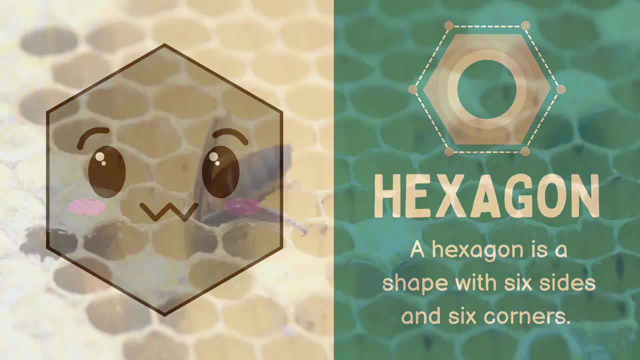 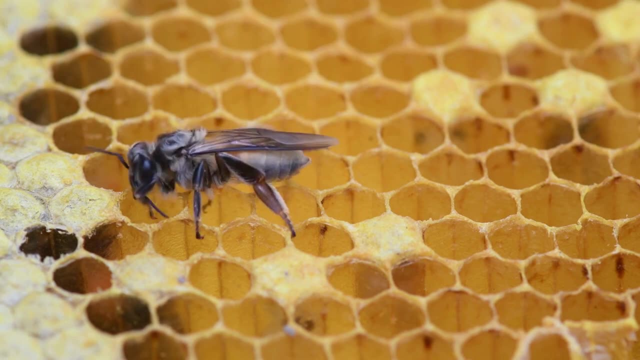 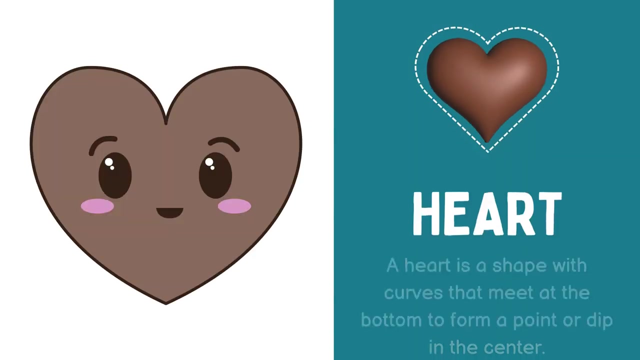 In hundreds of guards, fatters swell In behinds, busy In soccer balls, In crystals torn in all icy walls, A hexagon's alluring in fralls. In symmetry, it stands tall. Now let's speak of the heart shape, With curves that meet.